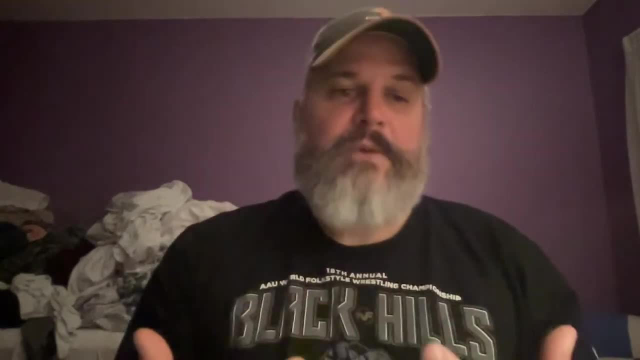 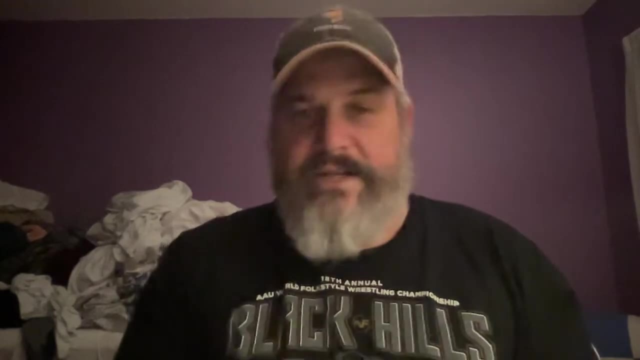 While looking at the photo, answer this question: How might population growth or decline change this human-built landscape? Okay, they'll jot down their answers, They'll discuss it as a table and then we'll just talk briefly about it, right? 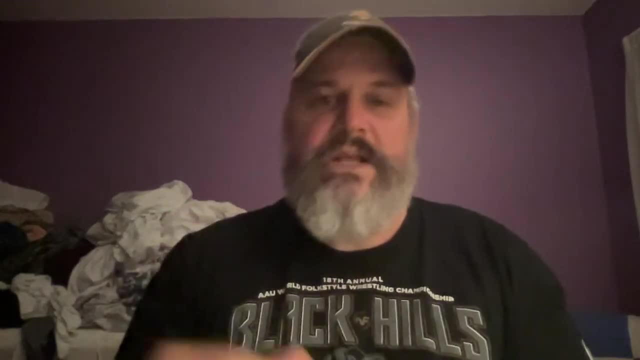 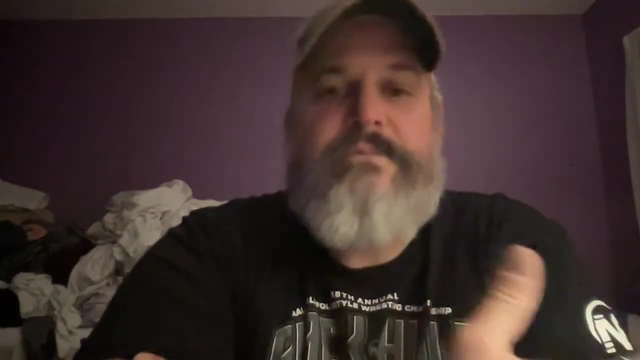 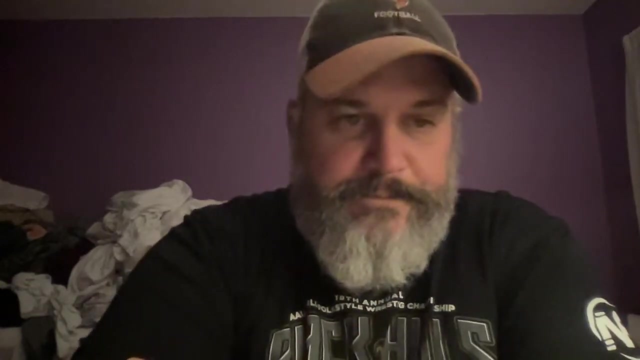 This is an opening to the lesson, the anticipatory set. See what they know, See where they're at. Okay, So how am I going to go about teaching about the patterns and the interventions, actions and things like that? well, i'm going to approach them with a discussion set to discuss. 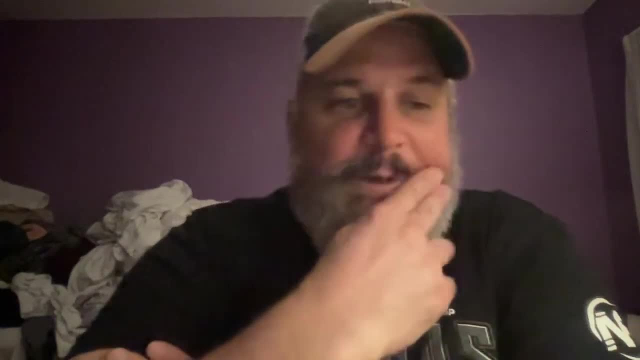 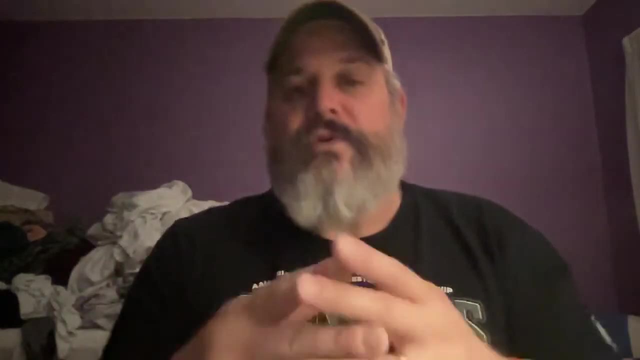 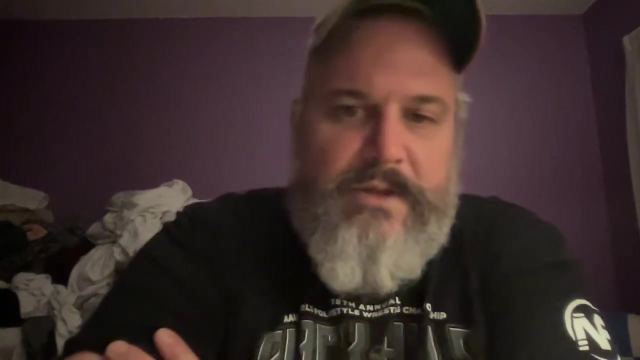 in groups as a class as we go through some of the material, okay. so i asked this, this question to start with, and i like to have them discuss it with one partner first and then as a small group, maybe three or four people tops. okay, you don't want to get too many more people um than that. 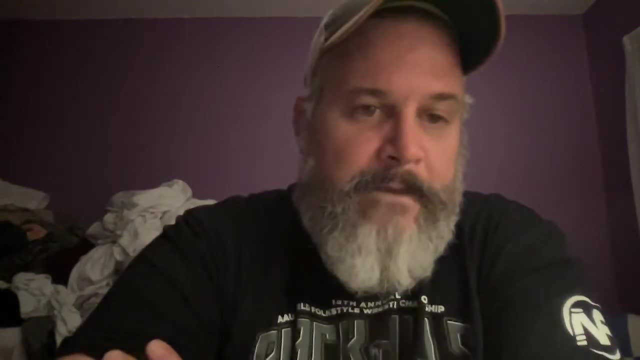 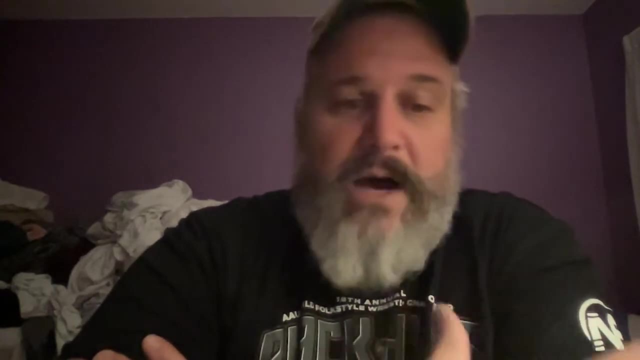 because then things can get awkward, all right. so, um, asking this question: where do you live, or where do people live and why? um, i'm going to moderate the activity. i'll walk through and, as i'm walking through, i'll throw out these other questions like: why do you live where you do, or what regions. 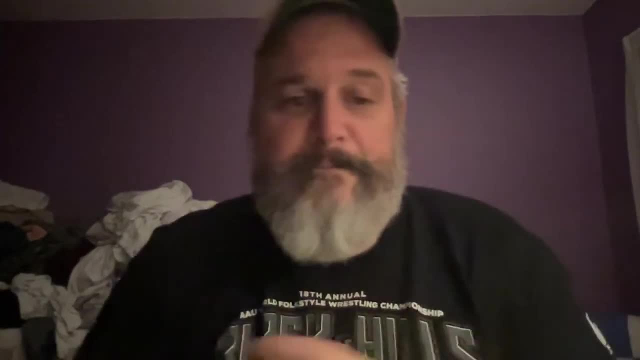 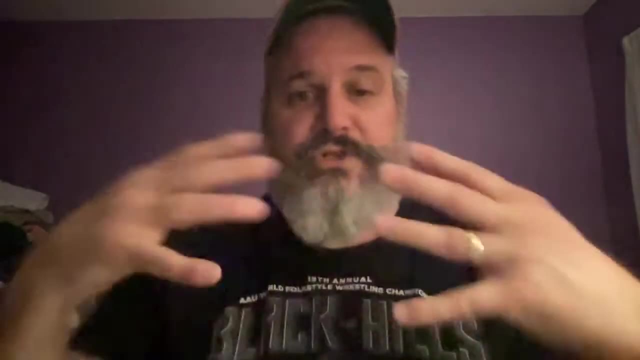 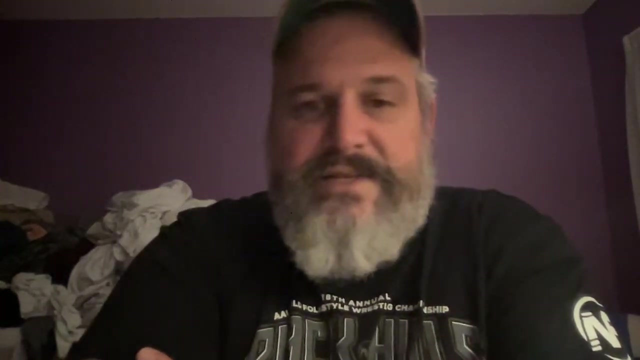 contain the world's- most of the world's- population. why is that? okay, so students will write down their immediate responses: um, they'll discuss with their partners and then we'll share out as a class. okay, um, and then they'll continue to review and tighten their ideas as they hear. 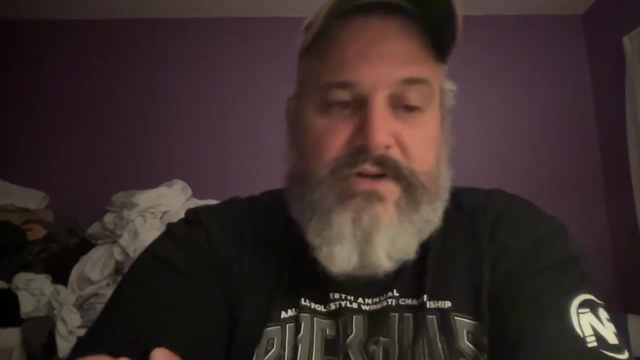 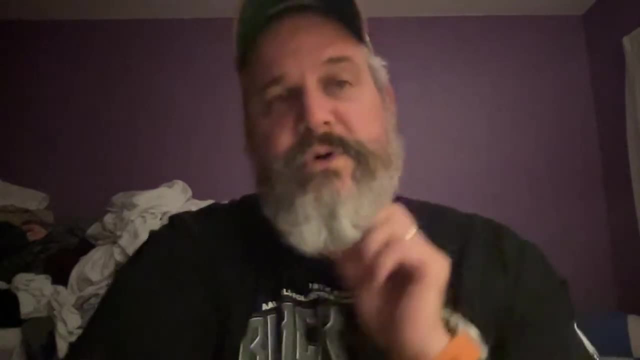 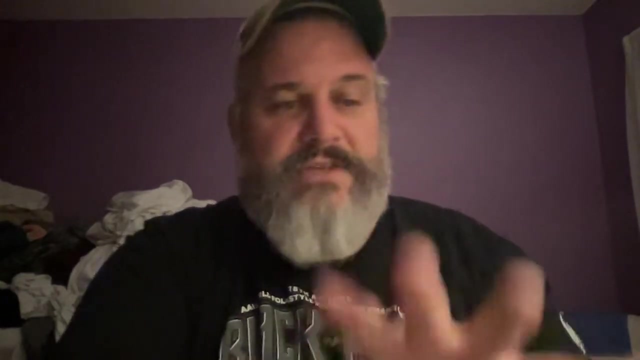 others responses. finally, in this instructional set we'll ask students to notice patterns in the clients classes responses and categorize them. okay, so that's the instructional strategies and we do this. i do this as i'm teaching the material. i'd love to ask questions as we're going through. 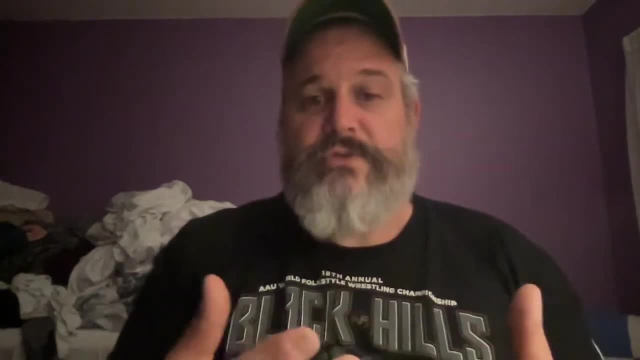 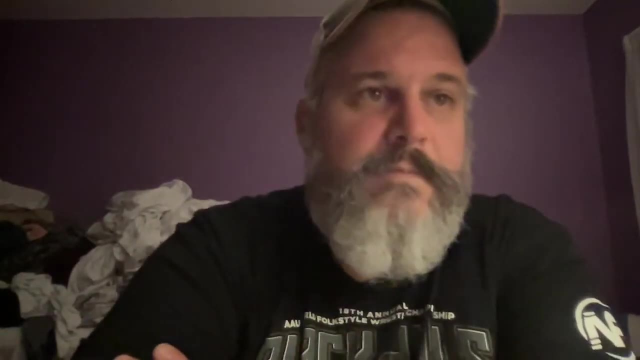 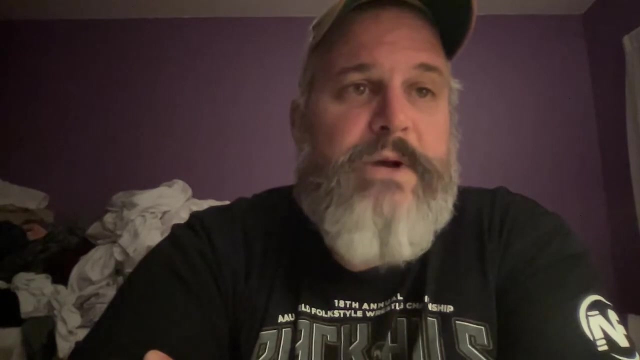 just to test the students. first of all, the students knowledge and second of all, what they're learning, and then thirdly, whether or not they're engaged. okay, so students will. they should have read the material before class, but i'll put them in groups. they'll be looking at the population. how, how? 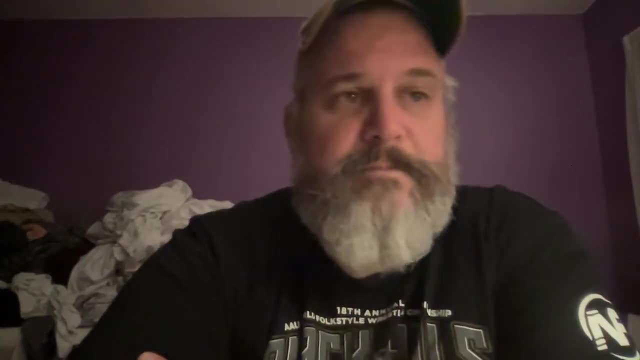 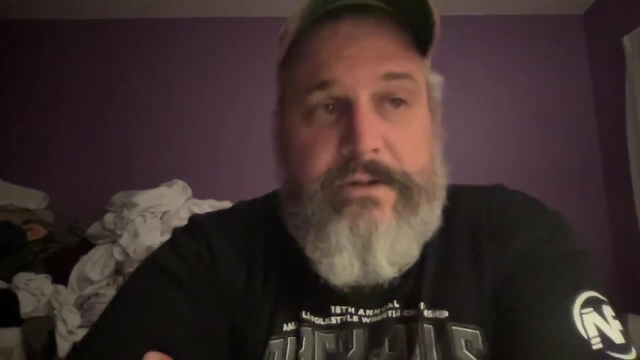 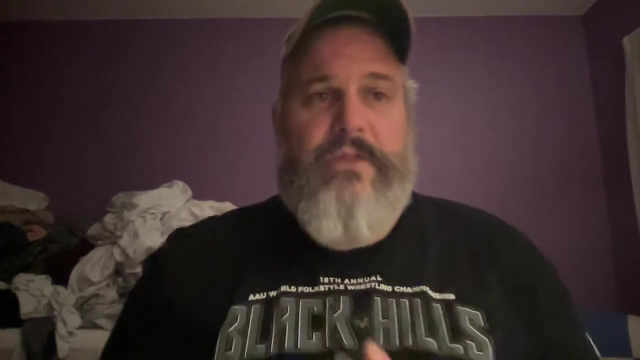 population migrates throughout the world and affects and the effects of that population migration. okay, so for the assessment for this section: okay, we will. students are going to complete. it'll be a two-person project. okay, it doesn't need to be more than two. okay, they'll research the practice of wet rice. 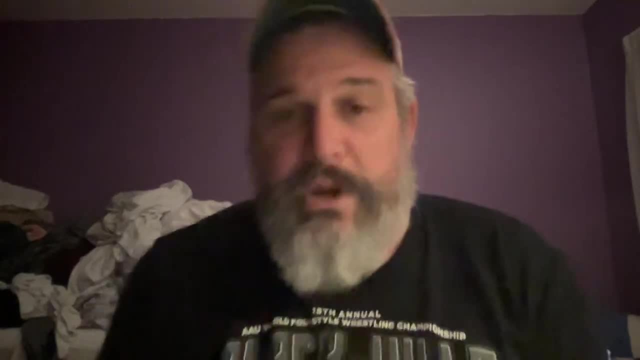 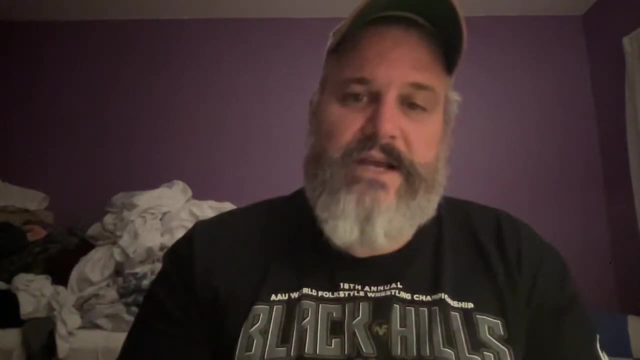 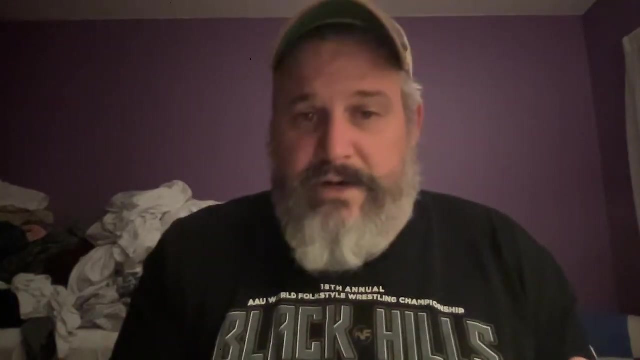 cultivation sounds super boring, but the key is getting them engaged in material and having them show how it ties into us today. um, just looking at our cultures right like in iowa, for instance, huge ag state, over 30 million hogs, corn, soybeans, you name it, we've got it. 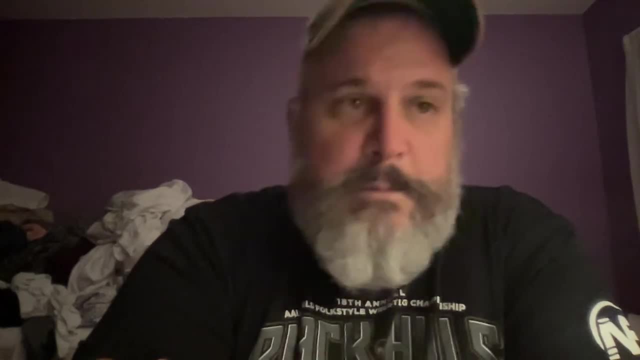 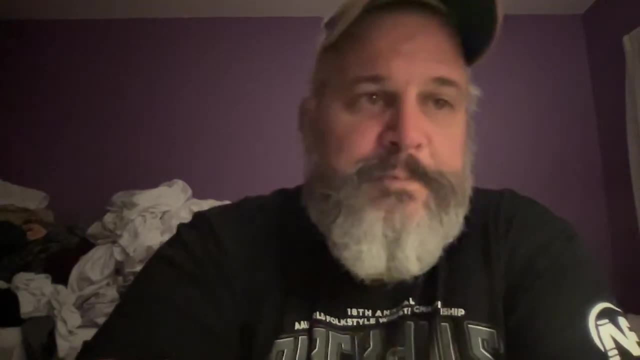 Okay, How do all those things infect the environment? Right? So with this, with this section of the world that we're looking at right here in the, in the Pearl Delta in China, they'll be looking at wet rice cultivation. They'll take, they'll need to take into. 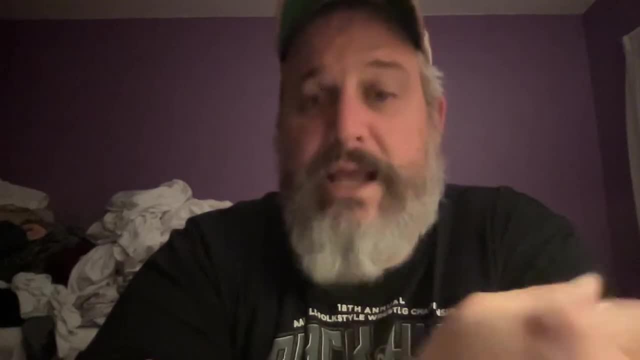 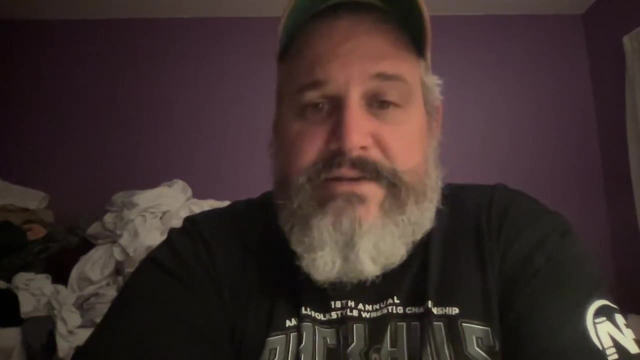 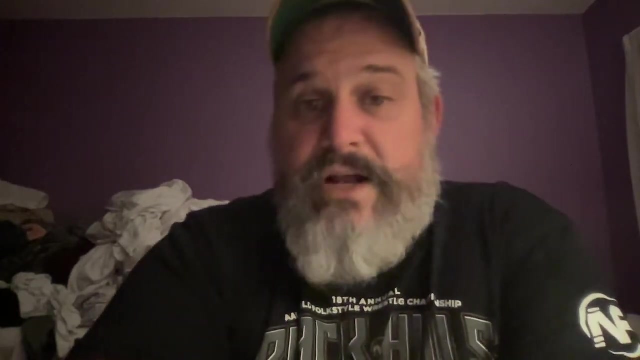 consideration how urbanization, climate and geography impact wet rice cultivation, And then they'll create a simple presentation or visual to summarize their findings. Okay, Specifically focusing on, like a geography lens, a human geography lens- Differentiation strategy. One of the things I love to do is give students voice and choice. 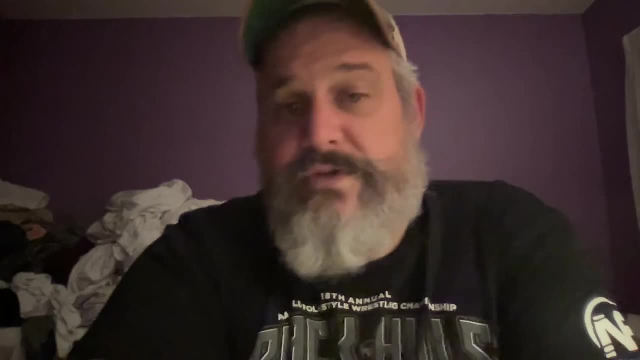 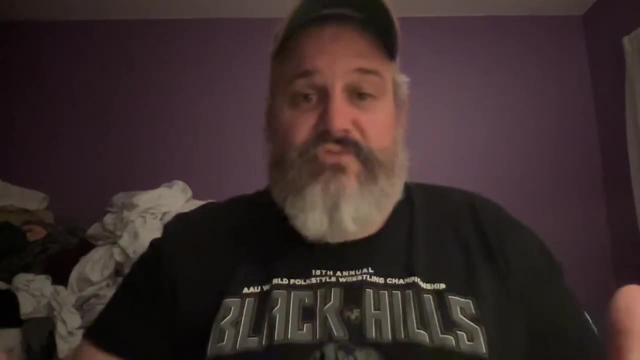 in how they present something. Not everybody's good with Google slides, Not everybody's good with PowerPoint. Some people are awesome at drawing. Some people like to do Powtoon and make things really super interesting. right, They have a choice in how they would like to present. 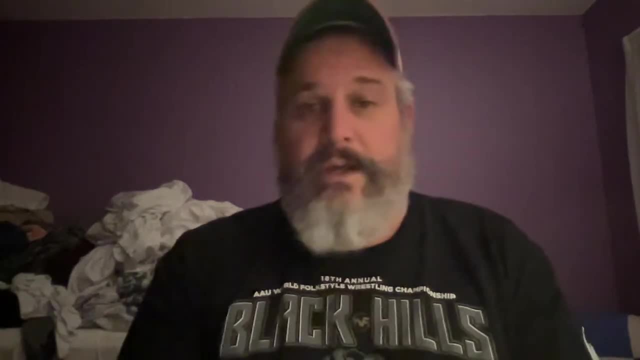 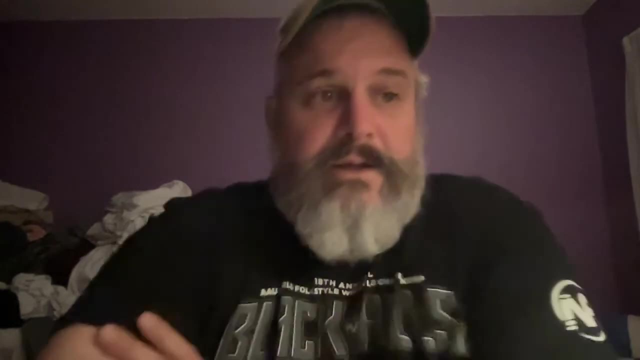 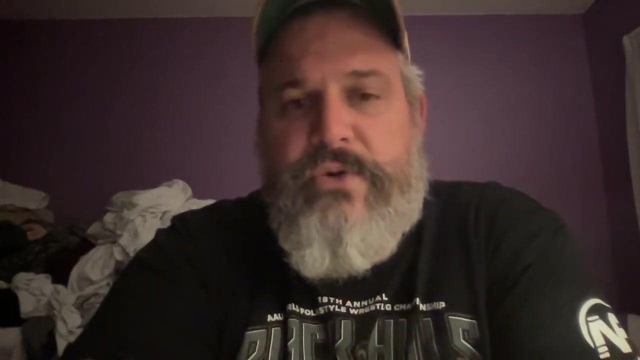 it. They can do a one pager if they want to, Okay, Which, by the way, other college professors out there- one pages are great and they're kind of fun to grade, Okay, And they can be higher order thinking as well. And then to close the, to close this, this specific lesson. 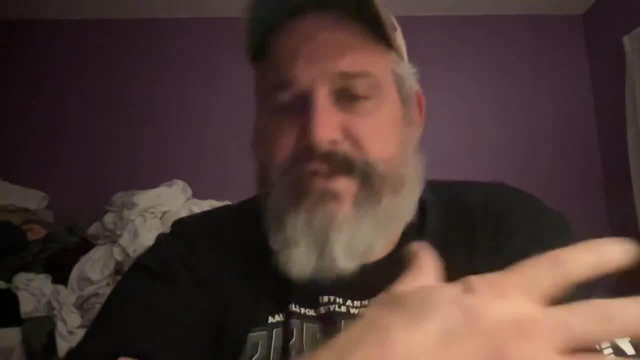 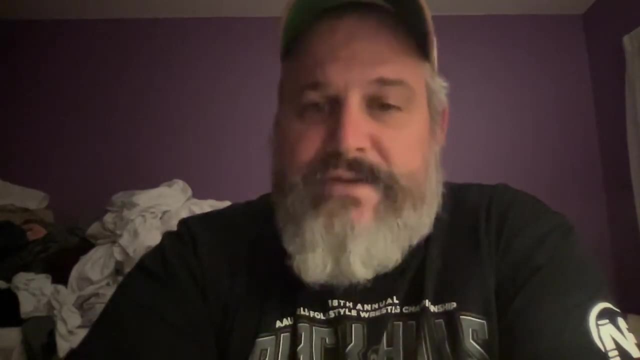 or topic out at the completion of the presentations because the students will present. we'll discuss the findings. right, Students will have to be paying attention throughout the presentations but we'll keep track of the findings, of what people- different people- have found. 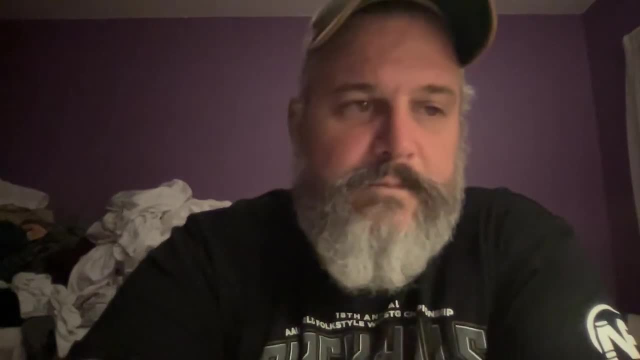 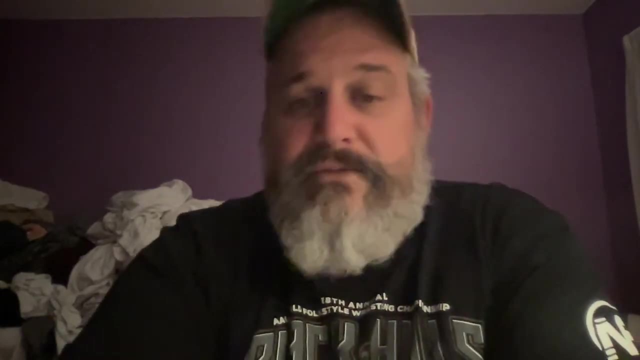 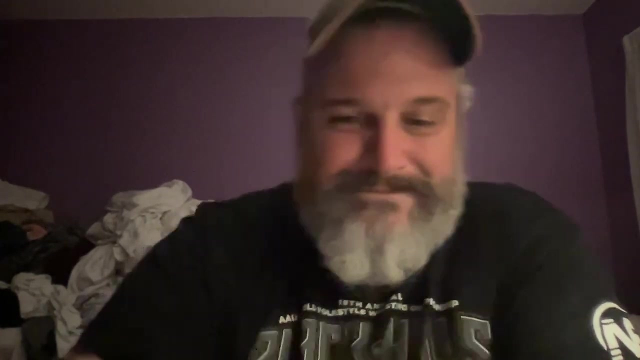 Because there's always different perspectives from different people. Look at the connections, Then we'll. finally, we'll look at the connections between population growth and migration in an area and how that could affect the environment and the economy. So I hope you have fun with this lesson. I know I will.